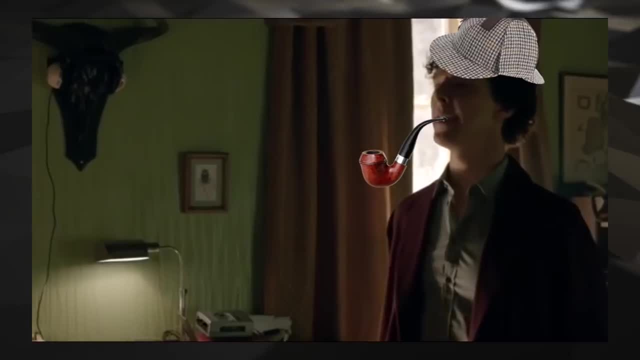 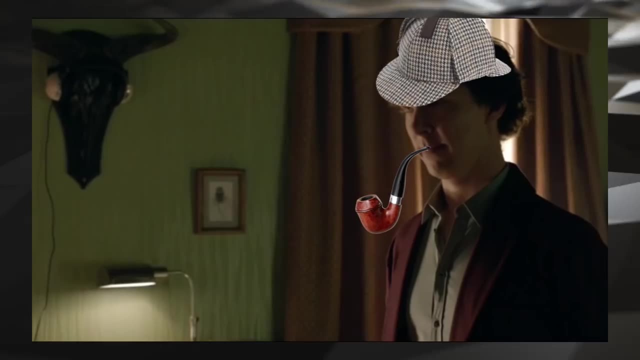 Hearse, where Sherlock and Mycroft were taking turns making deductions about a hat, and more specifically about the person who owned the hat, based on the hat itself. Well, if you don't, here's a short clip from that scene. Oh, and BBC, In case you want to claim one. 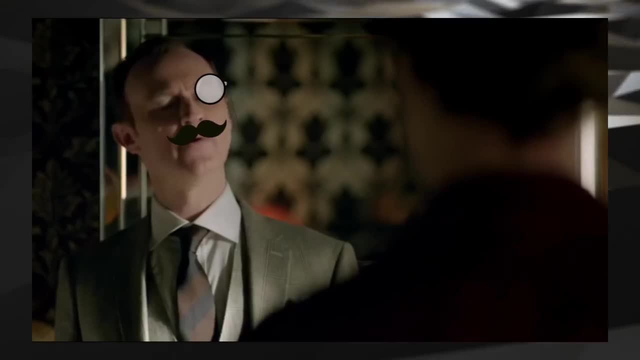 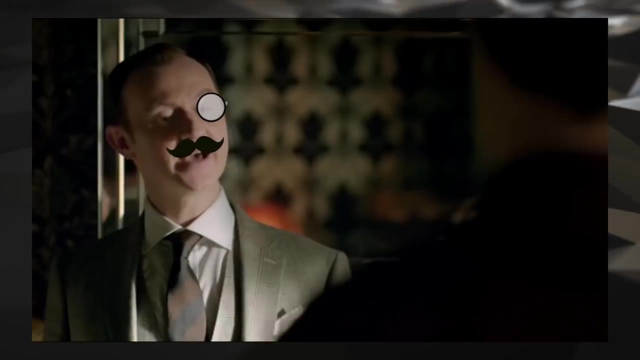 of my videos. again, the use of this clip is protected under the Fair Use Act as the use of this clip is transformative in the way that it is used to inform and educate. Love you all. And if that isn't enough, I've digitally added a deerstalker to Sherlock and a monocle. 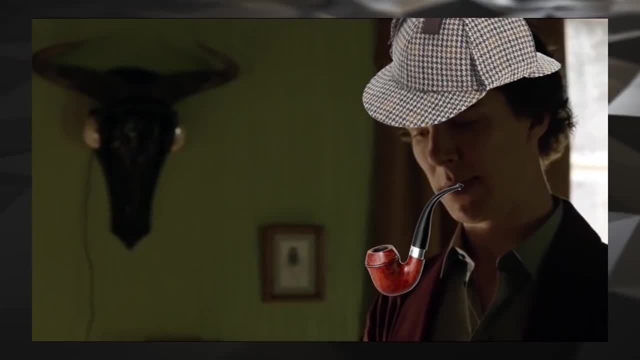 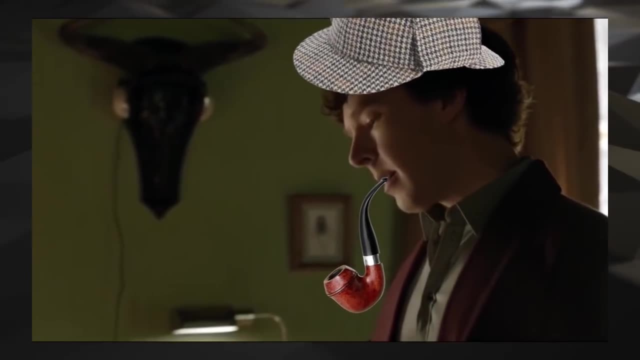 to Mycroft. so uh, there's that too. Anyway, now that we're all up to speed, I want to share with you a variation of this game that can help you train your deductive powers in a fun way. Now, this was my favorite exercise when I first got into deduction. I remember going 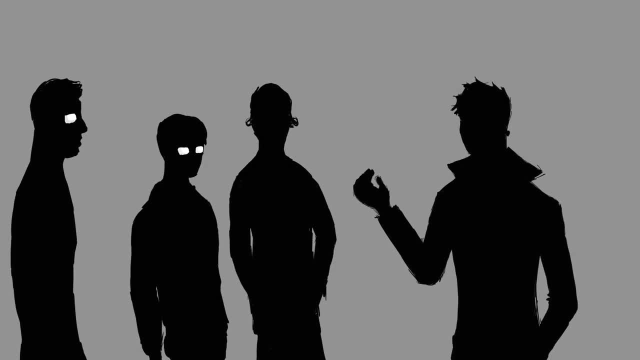 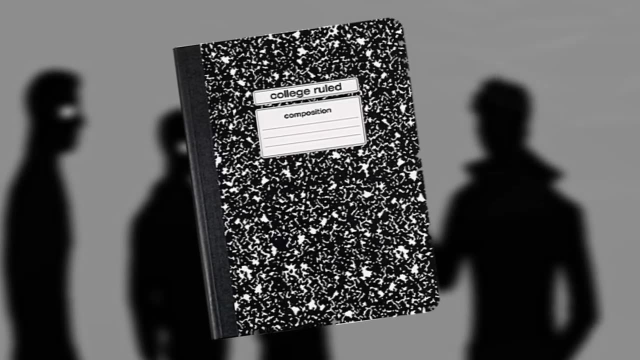 to school the day after seeing that episode and telling my friends who sat at my table in Geometry class about it. Then I proceeded to find a notebook that belonged to someone from the last class. I checked the name and it didn't belong to anyone in our period. Then I proceeded. 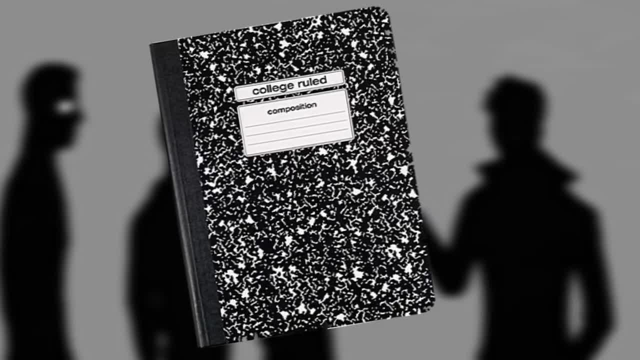 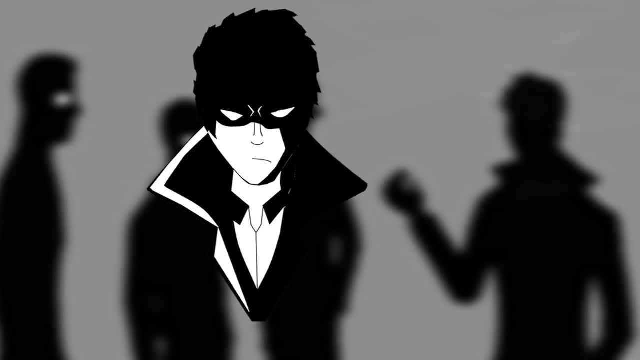 to make some deductions about it and I shared it with my friends to see what they could figure out. despite them not being super interested in deduction, They had fun A little. I think Maybe I did that plenty more times throughout the school year with various items and such. 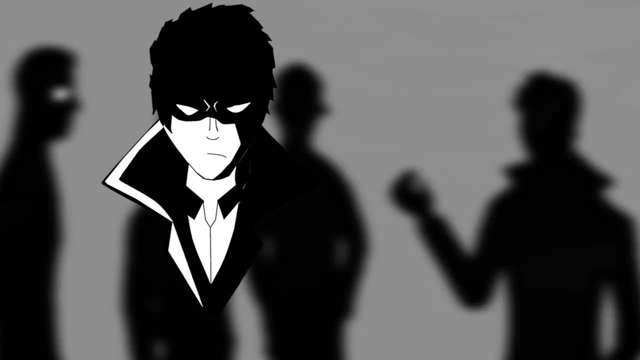 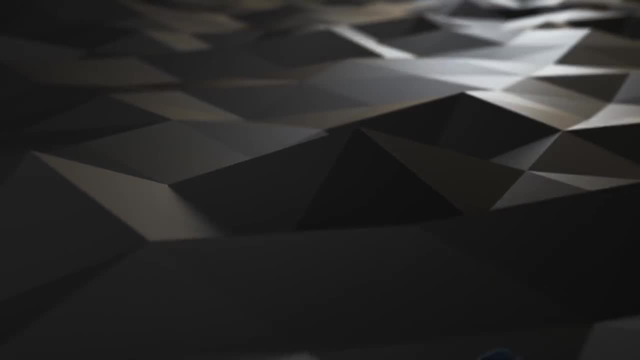 and it was quite fun. Then I started homeschooling and, you know, isolated myself, So that kinda ended, unfortunately, Regretting life decisions aside. in the instance that we see in this episode, you have two partners, both of whom are deductionists, making deductions about a hat. It's not like they're. 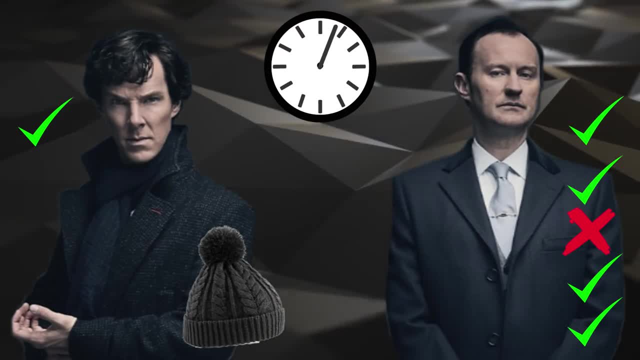 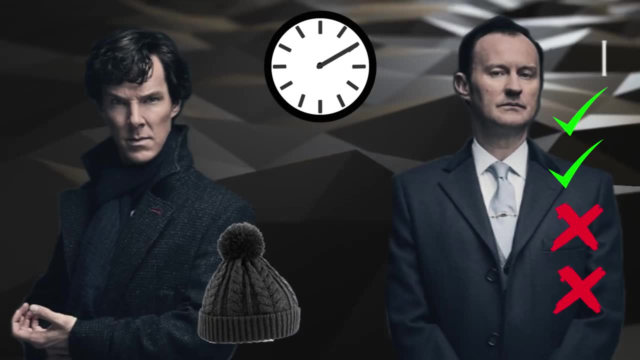 all the same. Essentially, whomever makes the most revealing and sensible deductions that fit the most data and comes to those conclusions quicker is the victor, And it also feels like that. it is broken into a round-based system with each pass of the hat. Now, if you 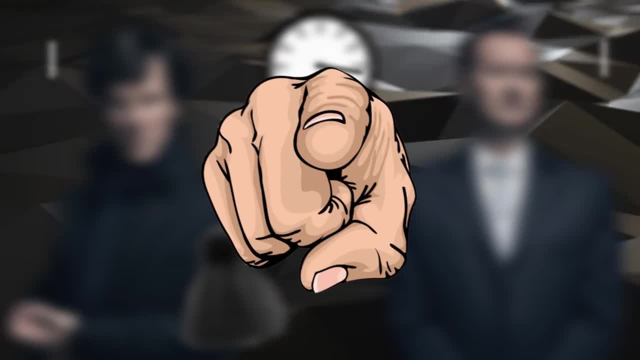 know someone who practices deduction as well. this is a great exercise for you. A bit of healthy competition will push you to do your best. However, for those of you who don't have a partner to compete against, I have a variation for you. 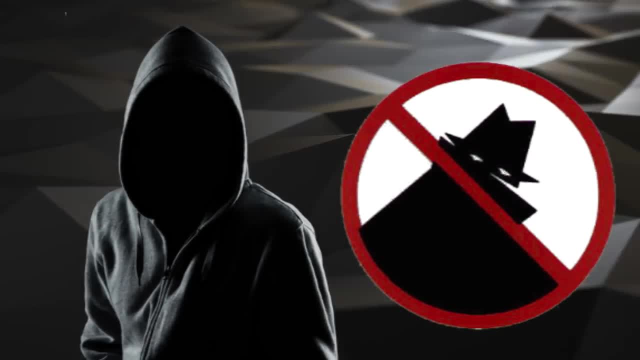 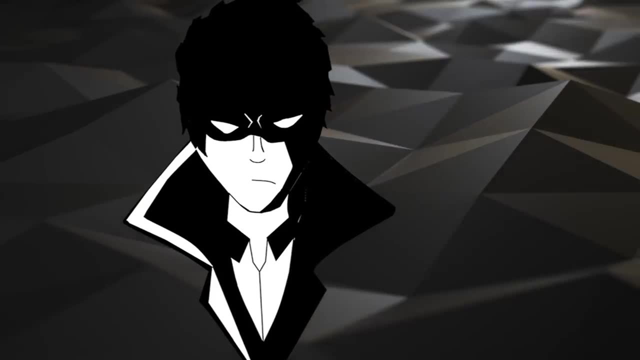 For this you will need two other people. They can be friends, family, strangers, what's ever, Although strangers make this a little bit more difficult. Have them decide amongst themselves, while you look away, who will be the one to give you something Then, once. 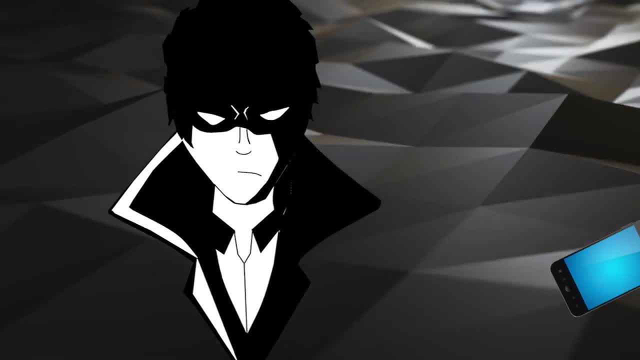 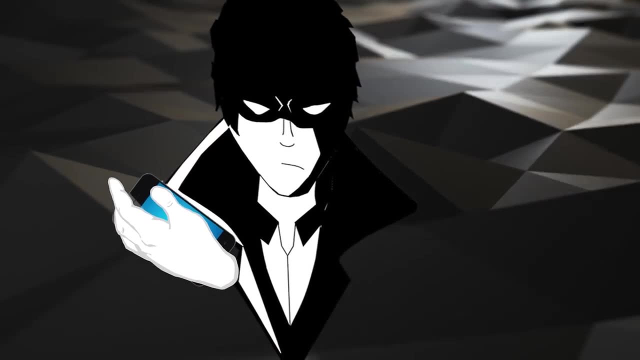 they have decided that person will take a personal item of theirs and place it on the table. Then they will tell you to turn around, Do so and take the item Now. make your deductions about the hypothetical owner of the item based on what you can observe. 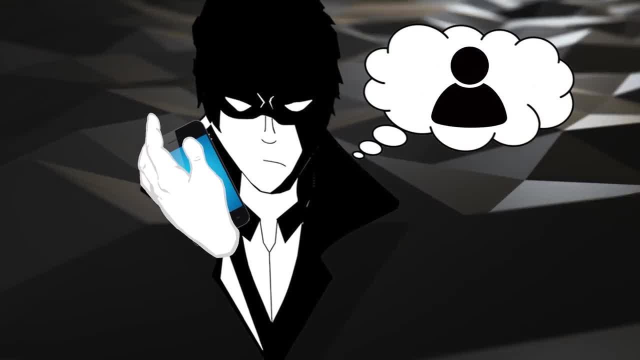 from the item itself. Build a profile essentially about the person who owns the item. Then see which of the two people your profile matches. So that's it for this episode. I hope you enjoyed it and I'll see you in the next one. 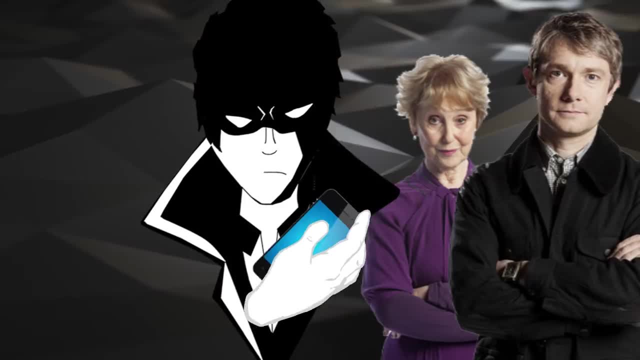 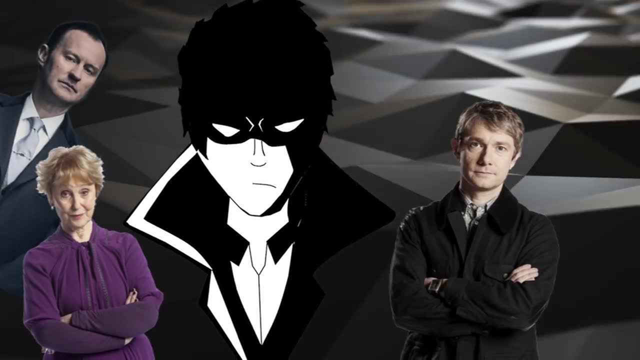 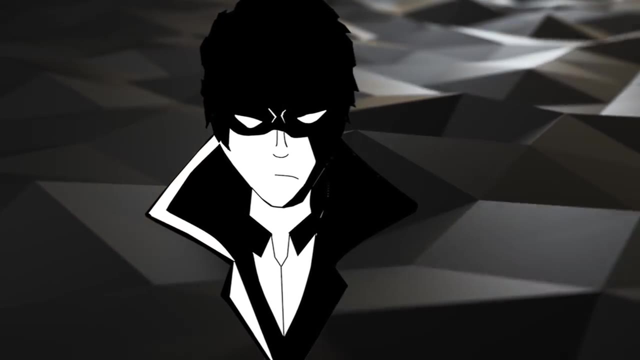 To increase the difficulty, you can always add more people to the game. You can have three or four or even five or six people in just one item. That is a lot of variables to consider. However, another way to increase the difficulty is to find two friends that 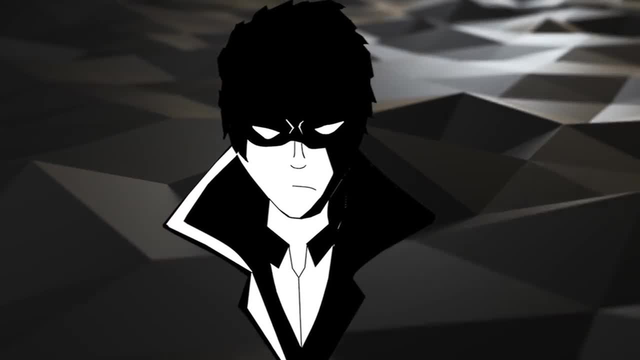 are very similar to each other, have a similar lifestyle or even live in the same house and abide by the same general schedule, such as two siblings. Their similarities mean that your profile based on the person you are talking to is the same as the person you. 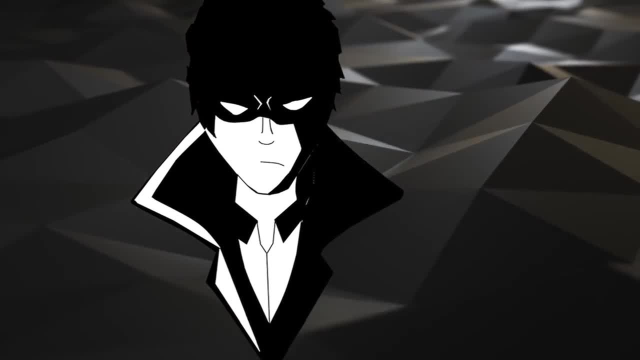 are talking to. So if your profile is the same as the person you are talking to, you will have to be more specific, because they match each other on all general accounts. Anyway, that's all for today. Play around with this exercise. see if you can put your. 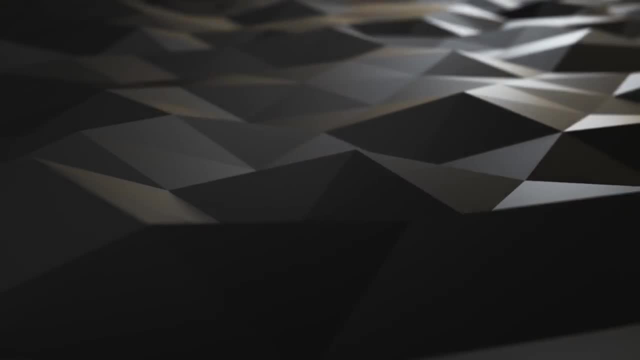 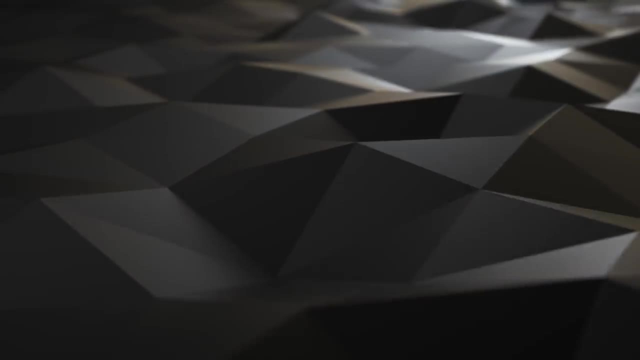 own spin on it and just have some fun as you train yourself to be a formidable deductionist. You know what? In fact, let's make this even more interactive For those of you who are keen. play this game with a couple of friends and film it, then send it to me via my Facebook. 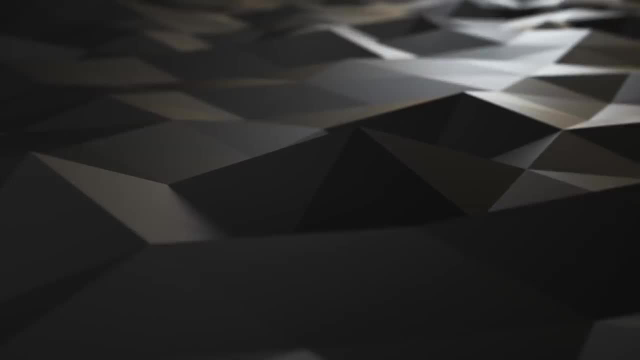 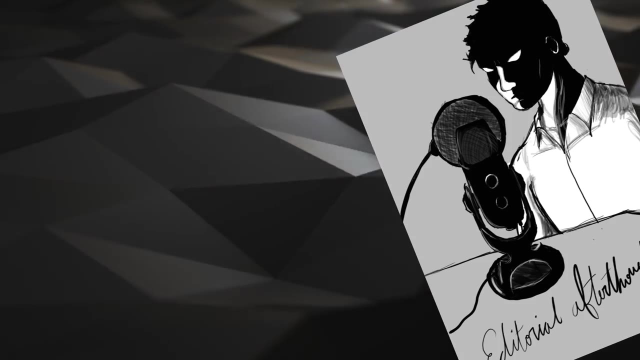 fan page or my email, both in the description. With that all you aspiring to- hang on, I feel like I should make some sort of reward or something for those of you who do this. Okay, how about this? Those of you who send me videos will have a chance to have your. 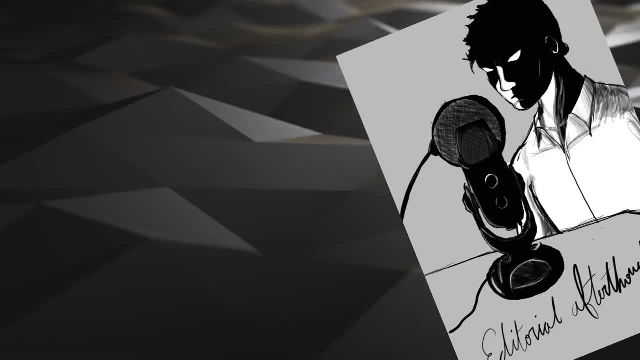 video featured on this channel. so if that sounds like something that you might be interested in doing, go for it. However, if you don't want the potential to be your face and deductions being shown to possibly 14,000 people, then maybe not something for you. Anyway, I look. 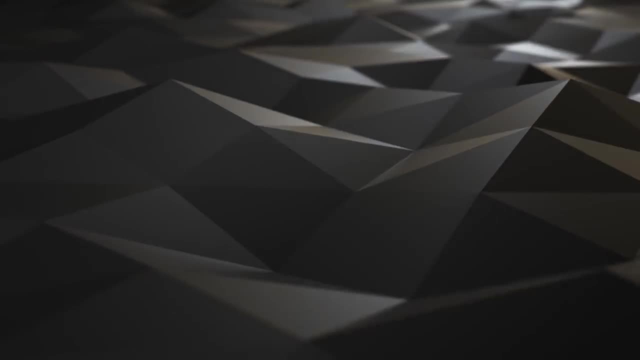 forward to seeing what you guys do. So if you're new here and you liked what you saw, be sure to subscribe. If you want to see more videos like this, be sure to subscribe to the channel. If you learned something today, give this video a like And, as always, I will. 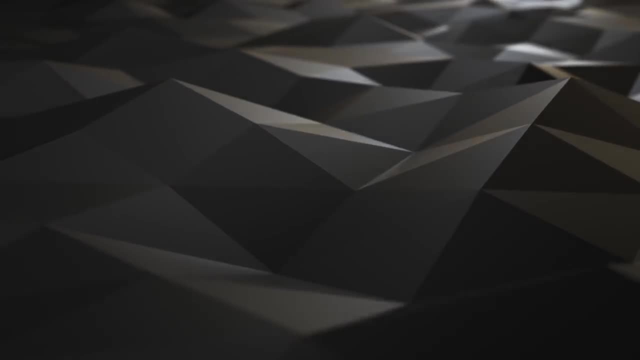 do my very best to answer any and all questions in the comments down below. Thanks for watching all you aspiring detectives out there. Arrivederci.